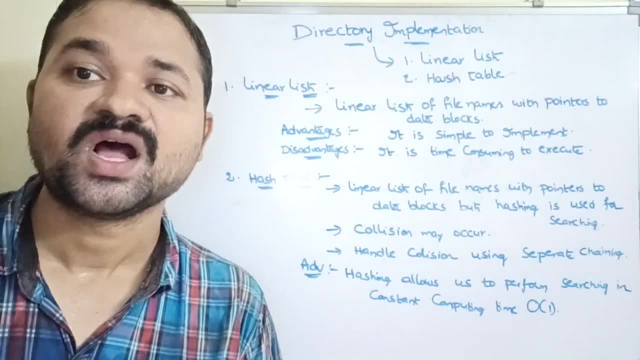 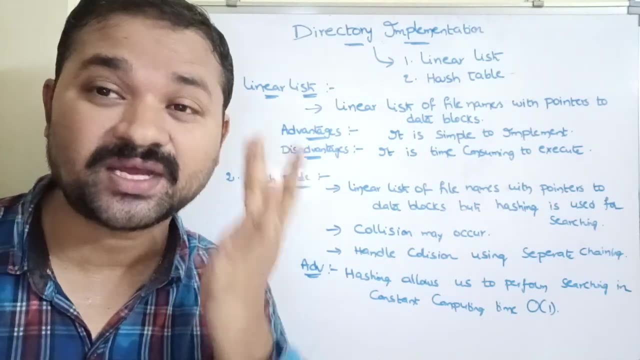 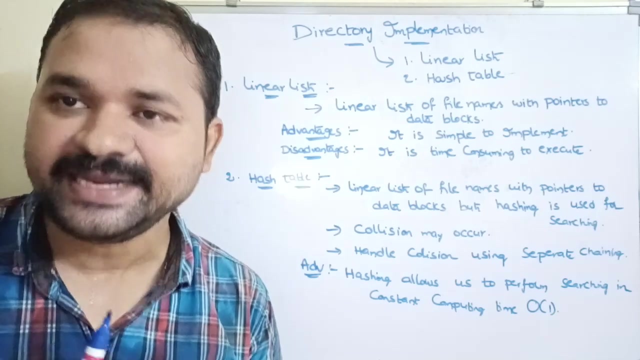 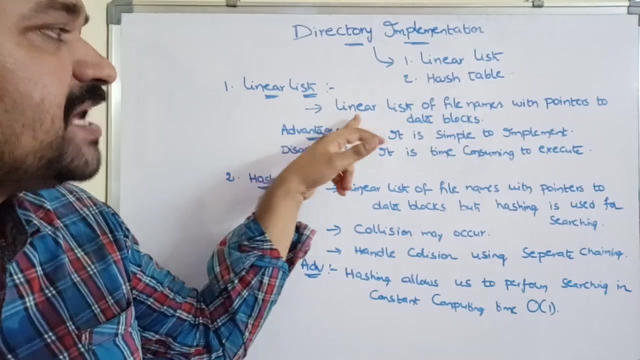 Now let's see about directory implementation. We know what is a directory. A directory means a collection of files. We use directories mainly to organize the files. There are two approaches in order to implement a directory. The first approach is linear list. The second approach is hash table. So let's see what is a linear list. So linear list means here we maintain a list of file names with pointers to the database. 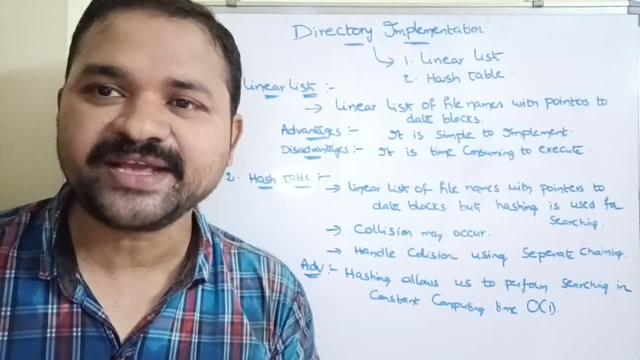 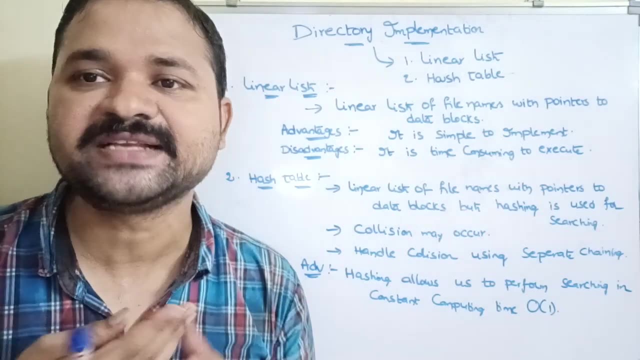 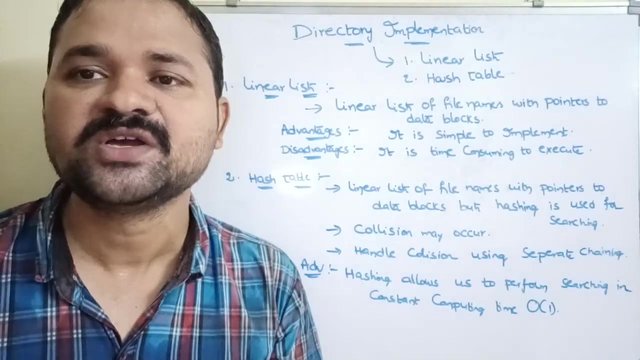 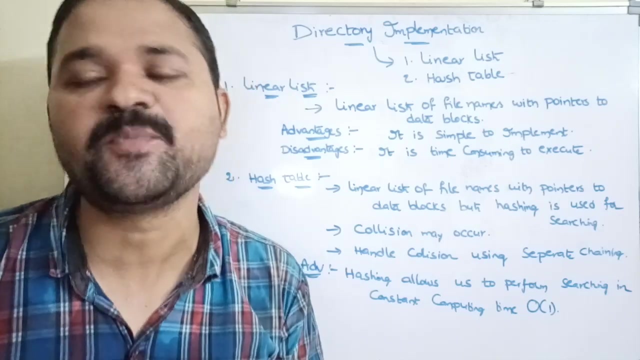 So we know what is a data block Here. the hot disk is divided into several blocks and in those blocks the file information will be stored. So we can say that the files are stored in the blocks, the data blocks, of the hot disk. So linear list means we maintain a linear list of file names and those file names points to the corresponding data blocks. 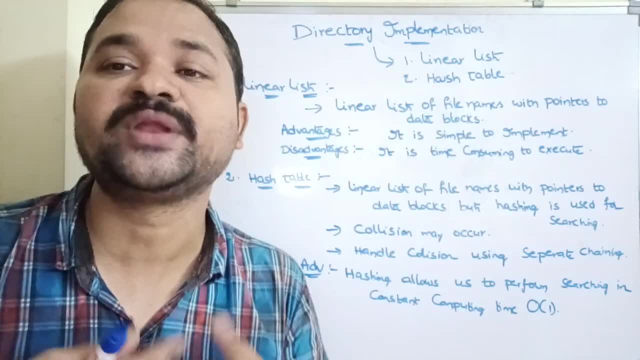 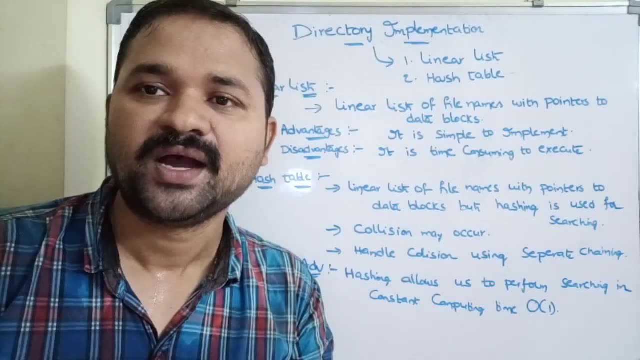 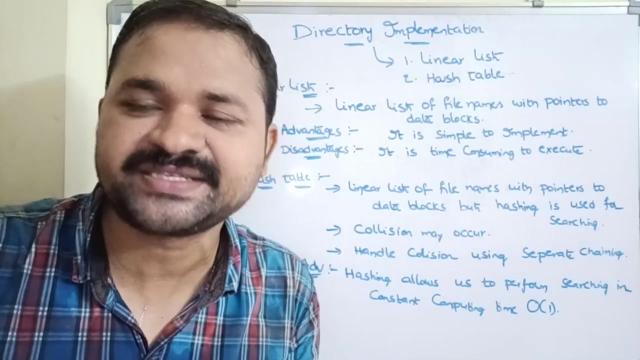 So here what will happen is, whenever we want to create a file, then first operating system will checks whether is there is any file with that name or not. for that it performs the searching in linear fashion or one by one. so let us assume that we have 100 files present in the directory. then first it search whether new file is same as the first. 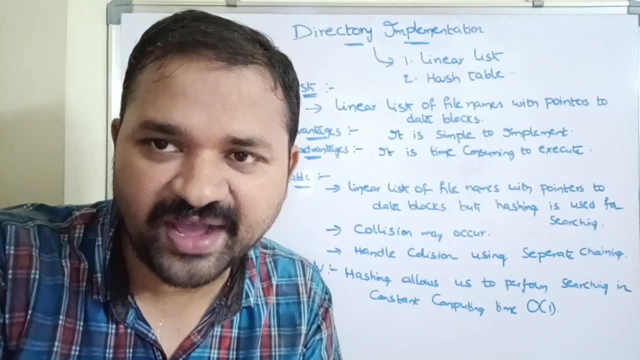 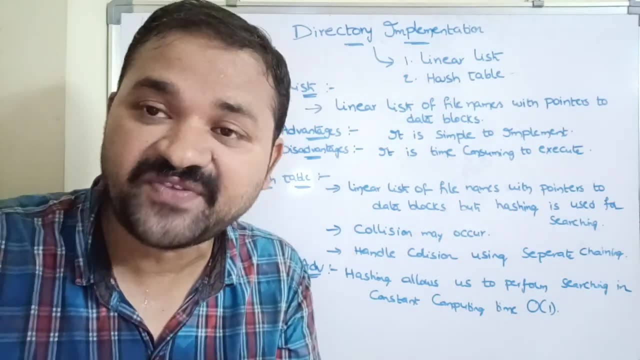 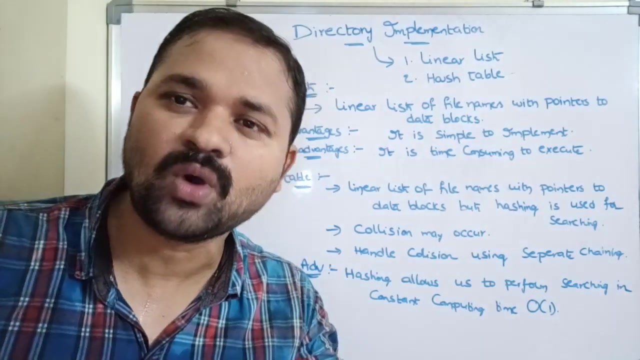 file or not. if it is not same, then it checks whether new file is new file is same as second file or not. next it checks whether new file is same as third file or not. so likewise it will for all the 100 files. so if the new file is not similar to all those 100 files, then it creates. 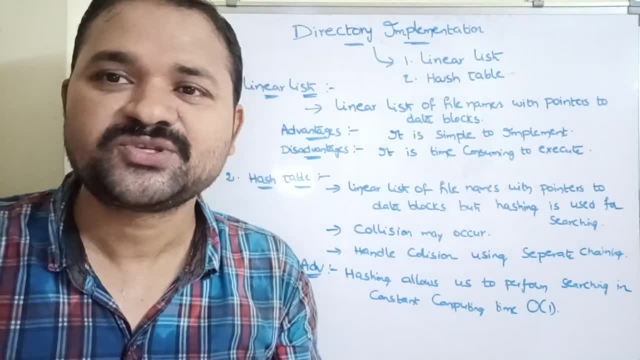 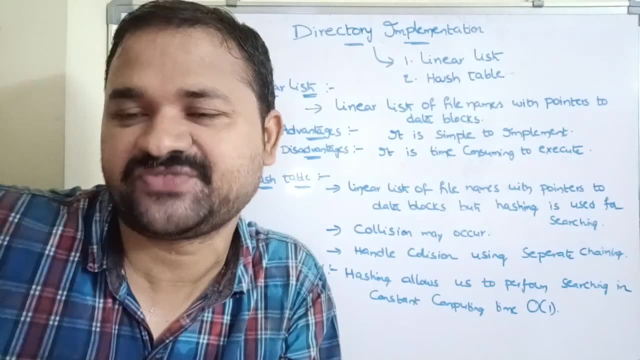 a file with that name as 101 file. so likewise for searching operation also, it will take small amount of time. we have 100 files, so it will check. it will search for the first file, next for the second file, next for the third file. so likewise for deletion operation. also it will take. 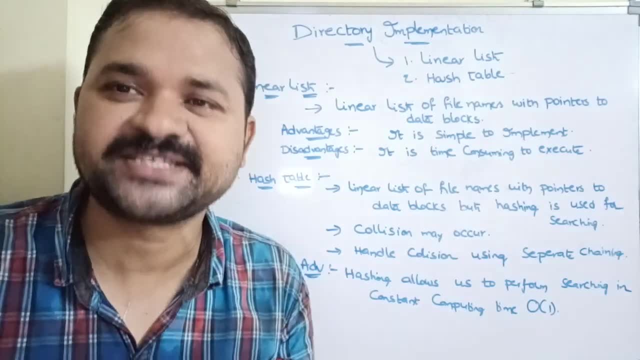 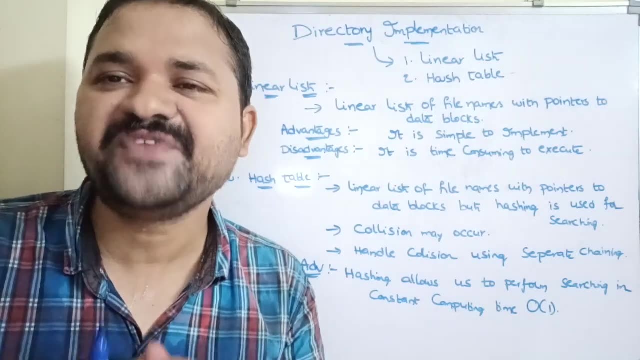 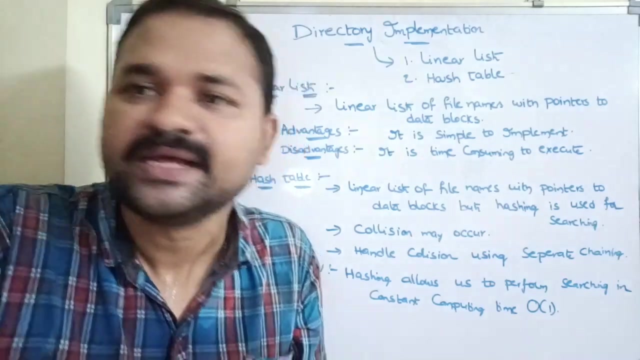 more amount of time. why? because all the files are set in linear fashion, one by one, one by one. so the major advantage of this approach is: it is very, very simple to implement this approach. so simply: we have to maintain a list, and that list points to an entry. that entry points to the corresponding data block. so it is. 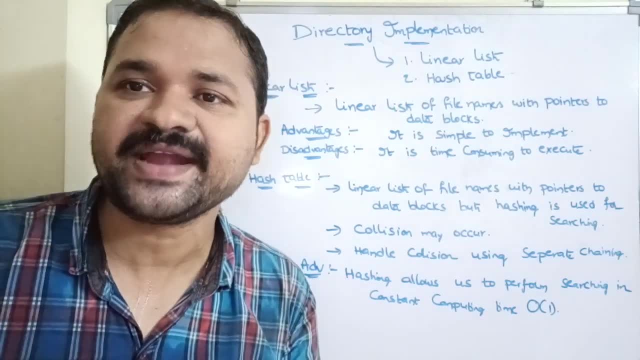 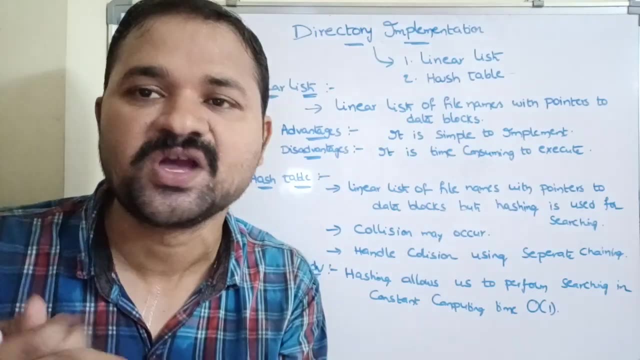 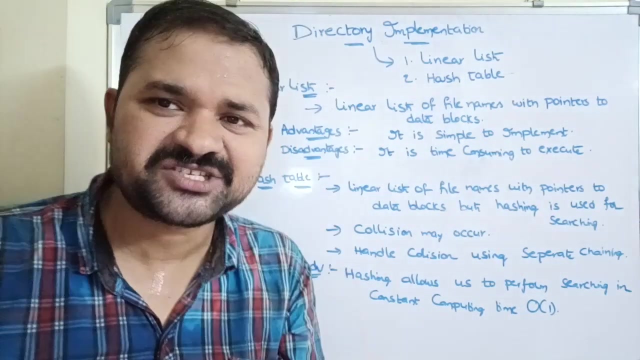 very, very simple to implement this approach. but the major disadvantage of this approach is it is very, very time-consuming process way, because here the searching is done in linear fashion, one by one. we can overcome this problem with the help of the second approach. the second approach is hash table here hash. 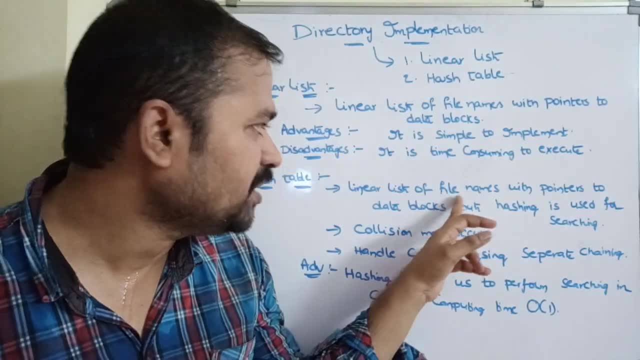 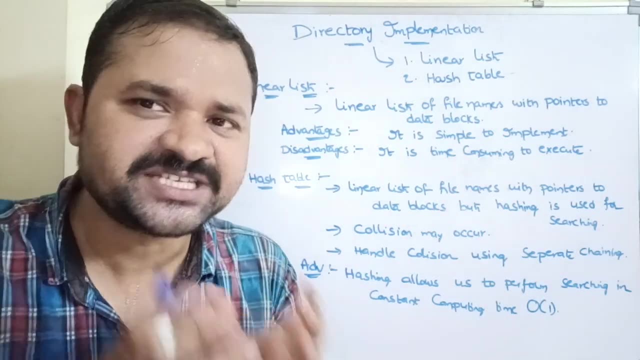 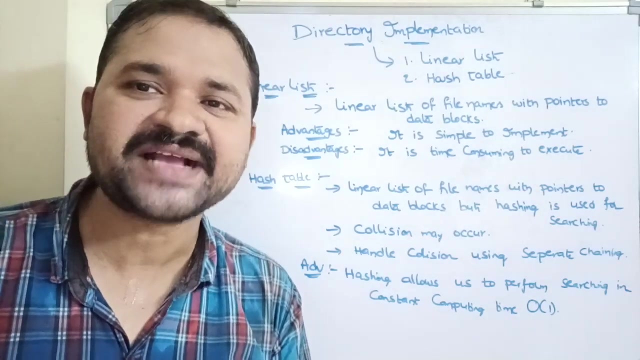 table means here also we are maintaining a linear list only so linear list of file names with pointers to the data blocks. but hashing is used for searching here. instead of using linear search, here we are using hashing technique. we know the major advantage of hashing. by using hashing we can perform the searching. 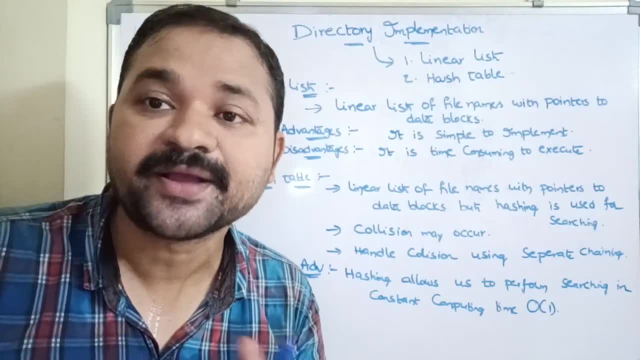 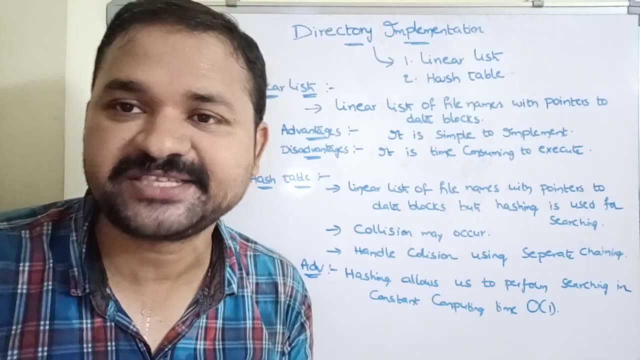 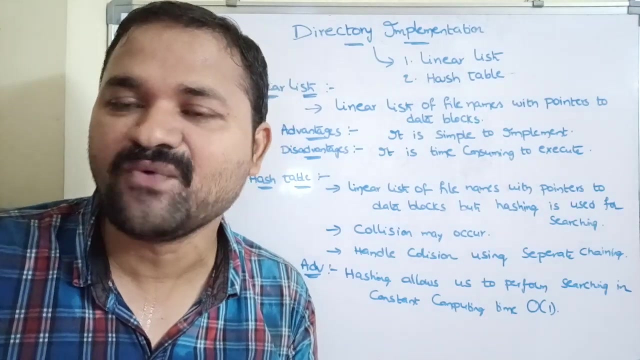 operation in a constant computing, in a constant computing time. so that means with the help of only one comparison we can perform the searching. if you take a linear search, then the worst case complexity is O. if you take binary search, then the worst case time complexity is O, whereas if 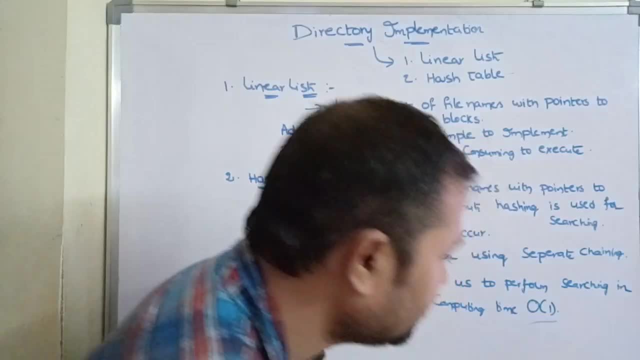 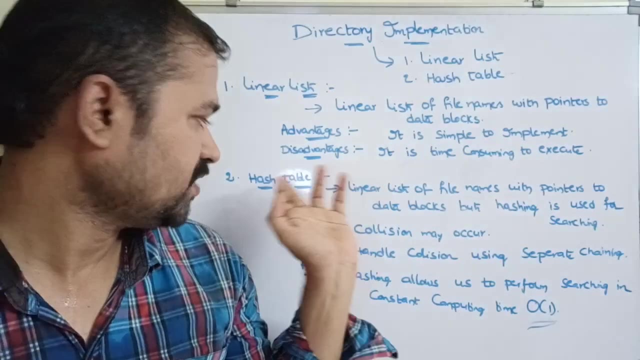 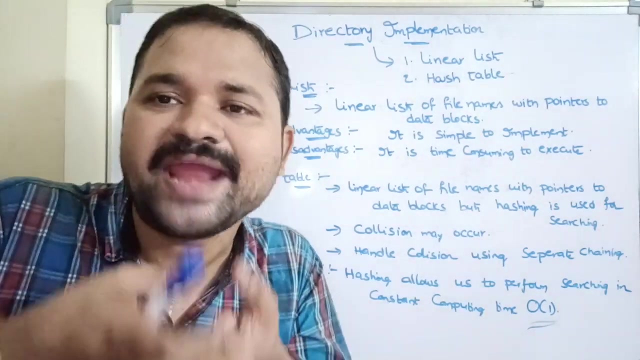 you take hashing, then the time. complexity is O. that means with the help of only one comparison, we can search for the corresponding file. so here, what is hashing paper here? here, also, in order to implement the directory, we are maintaining a linear list of files, and those files points to the corresponding data blocks. but here, instead of using linear search, 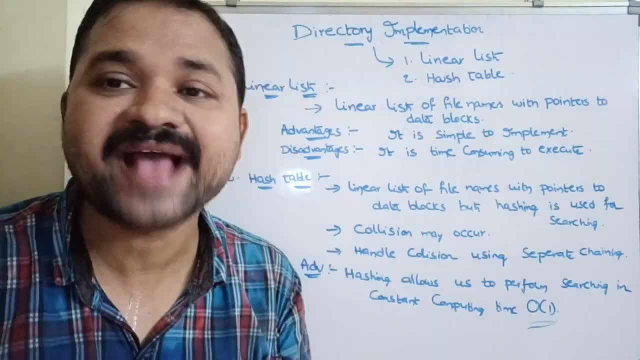 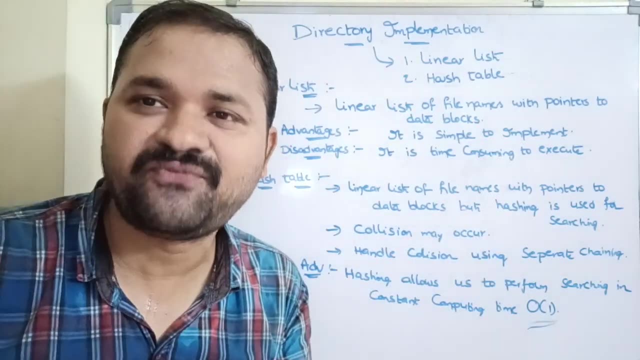 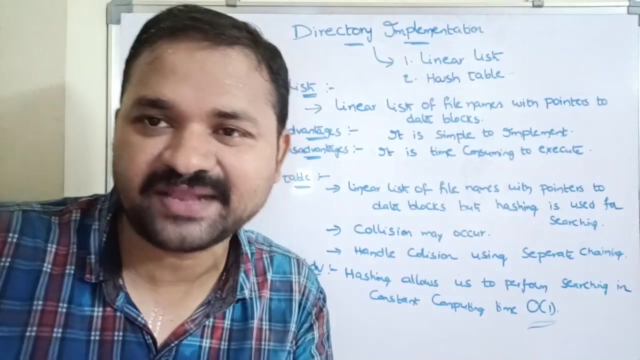 we are using binary search. i'm sorry, here we are using what? hashing technique. so let's see we know how hashing is applied here. actually, what will happen is every file has some identifier. whenever we create a file, then internally an identifier will be created at that file. so hashing is. 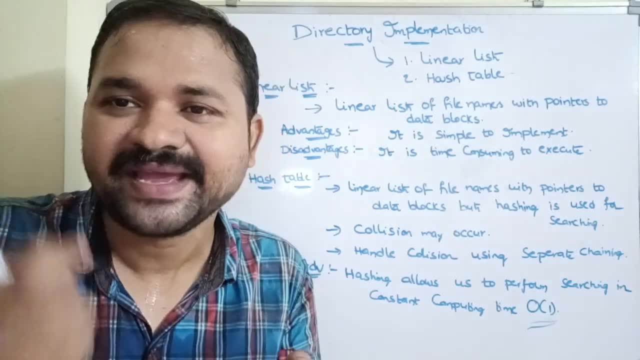 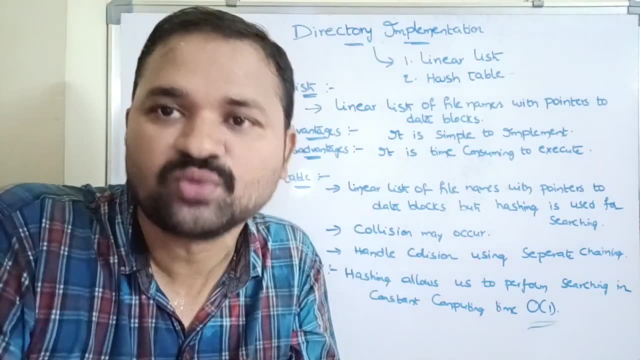 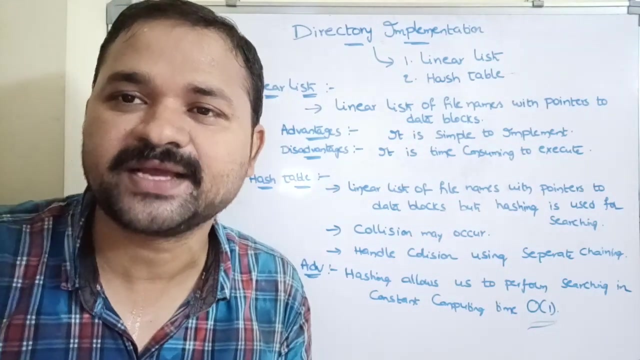 applied on that file. so hashing produces a hash value. that value is map to your entry in the hash table. so the corresponding value, the corresponding hash value, will be stored in a location of the hash table. but here the problem is that sometimes there may be a possibility that more than one key or 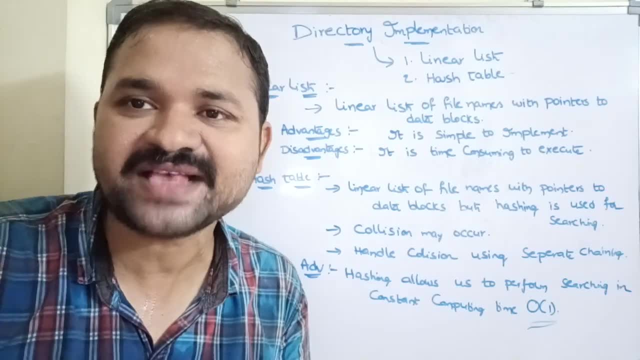 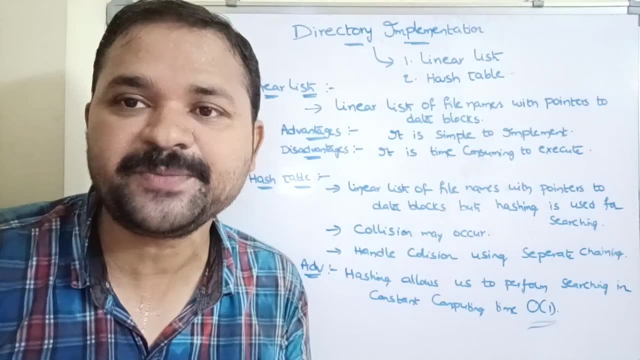 more than one value mapped to the same hash table. so in order to be able to create a hash table, you location of the hash table, so that situation is known as collision. so whenever we implement hashing, then there is a possibility that collision may occur. so whenever collision occur, then we have